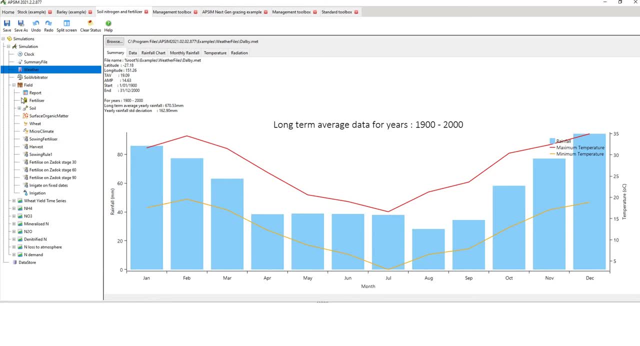 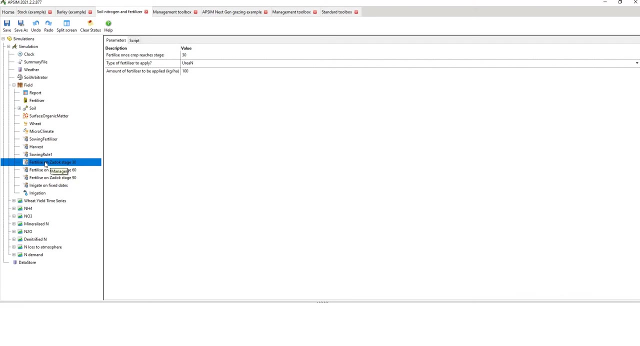 to adapt that. I've then dumped in a number of specific manager components related to fertilizing. so you there's a number of different ways you can fertilize the crop. you can fertilize based on crop stage, on a specific date, on sowing, for example. so you have this one here where you can add an amount of. 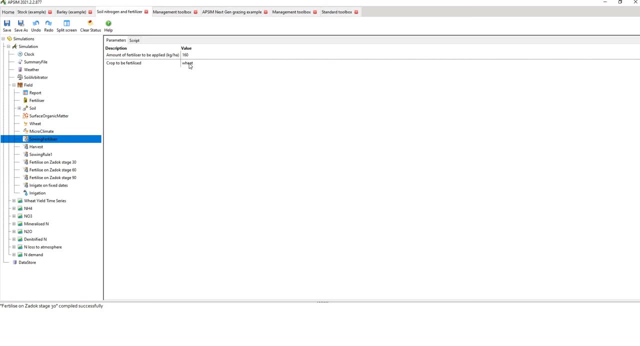 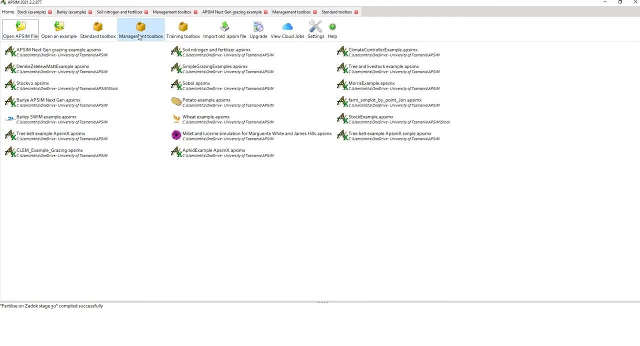 fertilizer on sowing, so it's adding 160 kilos of nitrogen per hectare to wheat. what I've done is I've gone to home management toolbox and in here you can see a bunch of different examples with which you can fertilize your crop. so it 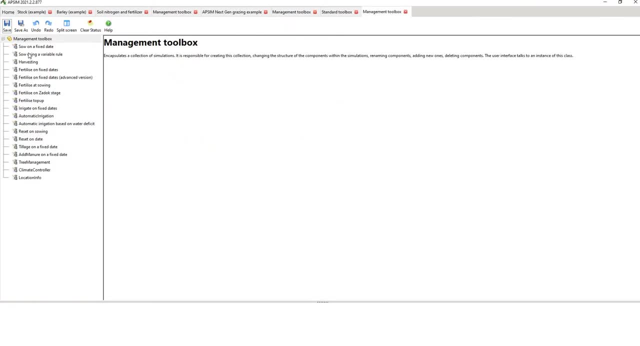 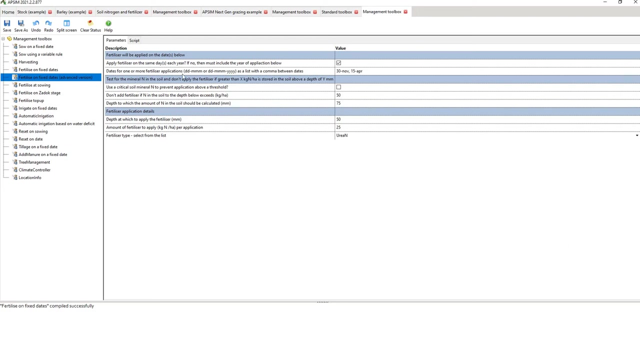 always takes a little while to open because it's going to the toolbox itself and it shows you what you can essentially do. if you click on them, it brings them up. you can fertilize on a fixed date. that allows you to nominate your fertilizer. there's a, an advanced version of that- fertilize on a fixed date, and so in this, 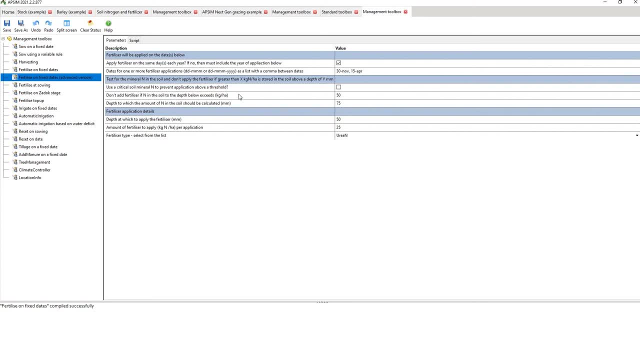 you can apply fertilizer at multiple dates. you can decide not to apply nitrogen if it goes above a certain threshold. you can add fertilizer below a certain depth. you can calculate the amount of nitrogen in the soil. you can apply fertilizer specific depth and then you can determine what type of fertilizer you. 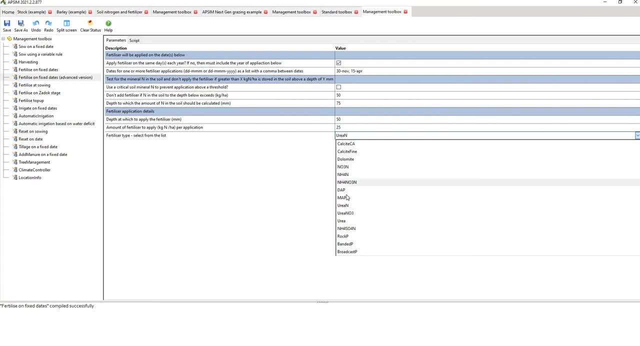 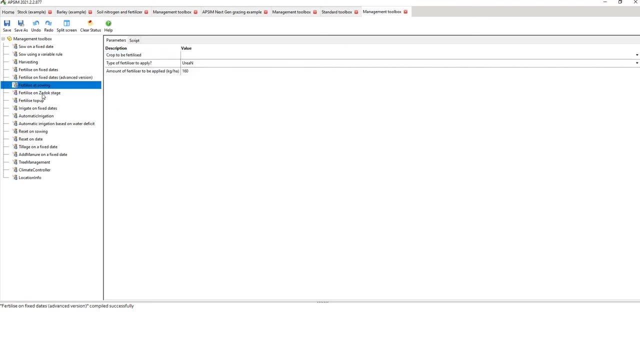 want to add. so you can add not only nitrogen, the AP or MAP, urea N, you can add different types of phosphate as well as calcium. so what you do once you've selected on your fertilizer regime- so there's other management regimes in here, but on- so you can do at sowing, at Xadox stage, or you can top up to a specific 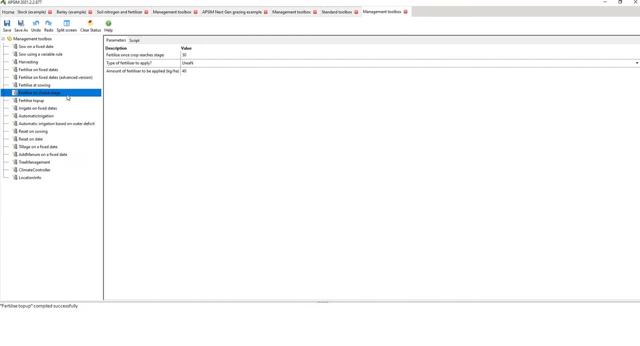 level in the crop. so I've got this one here. I've copied it: fertilize on Xadox stage, which means crop development. I went back to my example and then I've right-clicked and I've pasted it so and then, once it pastes, you'll see it pop up. 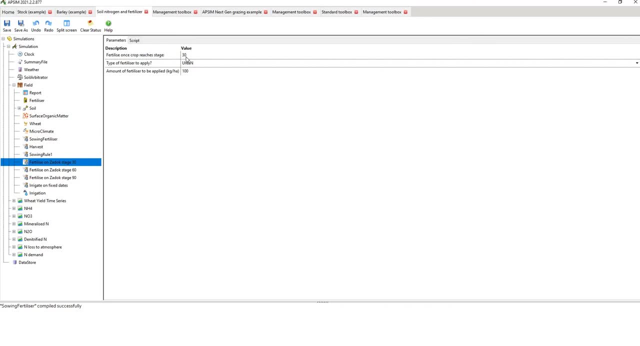 here. then you nominate which date, which, which stage with which you want to fertilize your crop. you tell it the type of fertilizer to apply. so that's going to apply straight urea nitrogen rather than urea per se. so urea is 50% nitrogen. 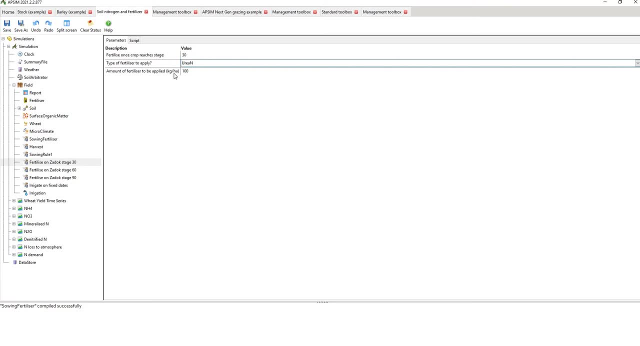 so if I apply a hundred, it's going to apply 100 kilograms of nitrogen per hectare. if that was just urea, it would apply 50 kilos of nitrogen per hectare, or technically 46, because urea is 46% nitrogen. so you, you come along and I've 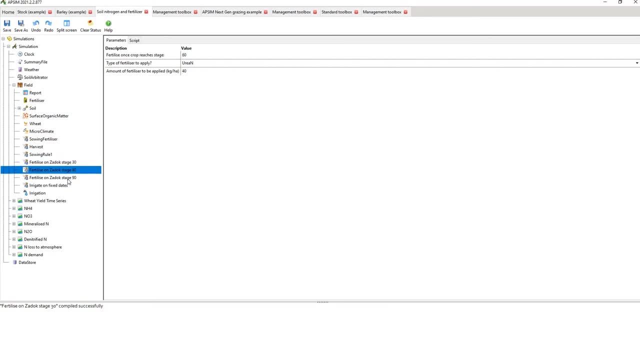 I've said: okay, well, I want to apply it at Zadok stage, 30 at 60 and at 90, at 30. I'm going to apply 100 at 60, I'm going to apply 40 and the same at 90, probably. 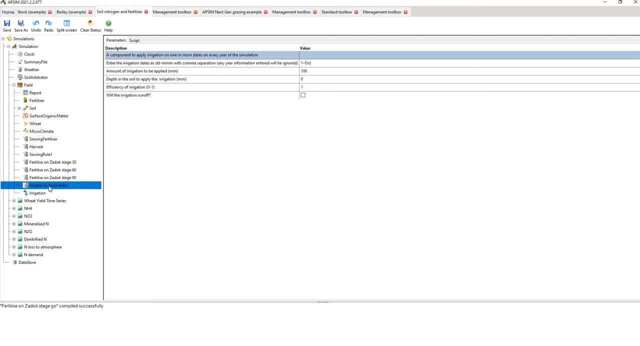 won't do much at 90 because it's already mature, but we wait and see you. I've also said that on the 1st of October, which in the summer season in Australia starts to get dry, let's apply 100 millimeters of irrigation just to. 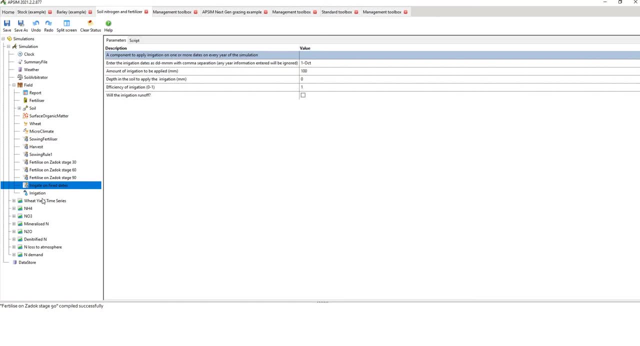 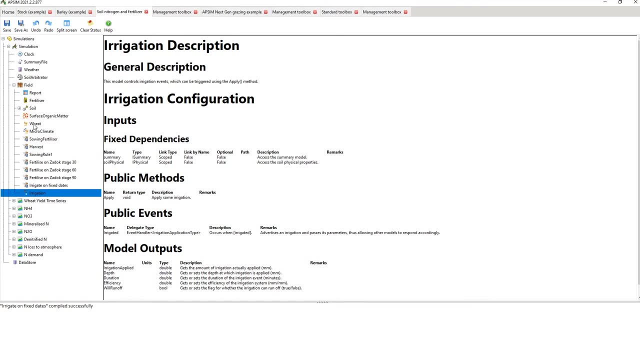 give it a water. and I've said a hundred percent efficiency. just for the sake of illustration, I've put in this irrigation component so that's so that Apsium actually waters. if you haven't got that in there, it'll give you an error, it's. 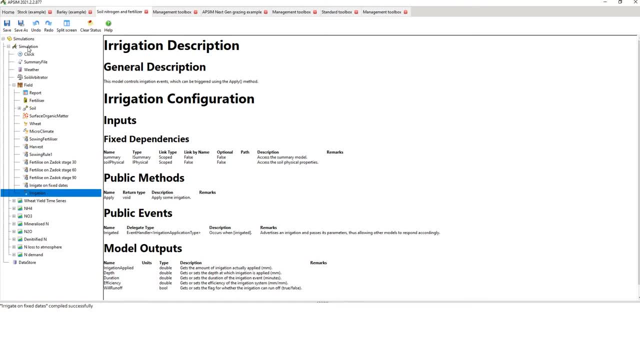 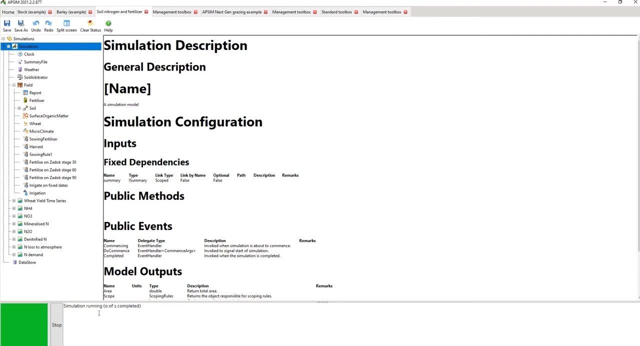 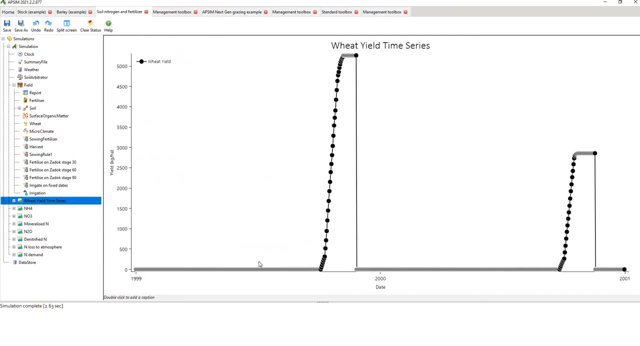 the same as the fertilizer thing. now we've got a number of graphs. so what I did then is I I put those in, I went run and hopefully you see it running here without an error. then what happens is you've got your yield, so it's showing you you obviously had a lot better year. 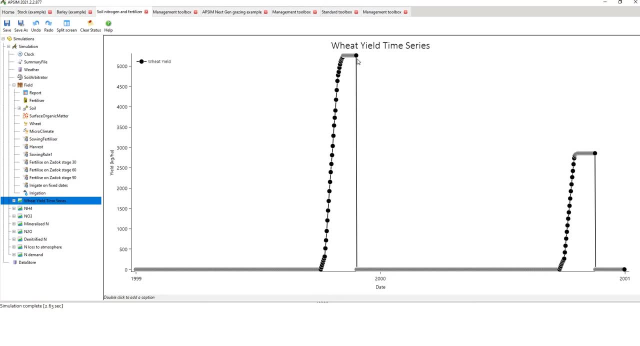 in the first year compared with the second. so in the first year we got a yield of about five ton per hectare, the second year about three ton. then I've put in a heap of nitrogen output graphs, so this one here is ammonium, which is the first. after nitrogen is hydrolyzed is the first step in the nitrogen cycle. 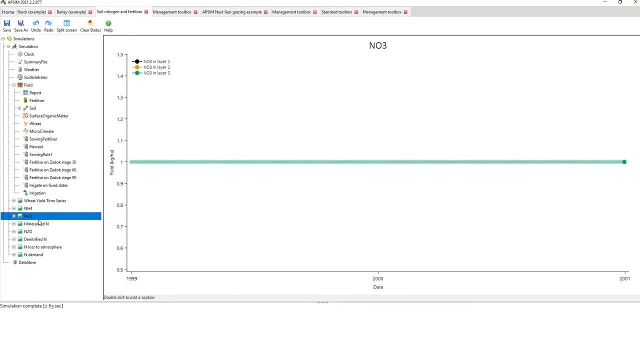 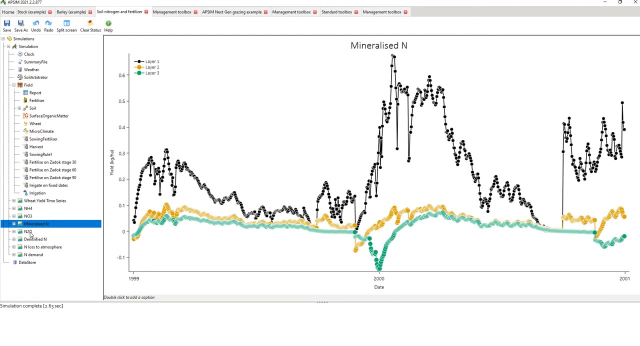 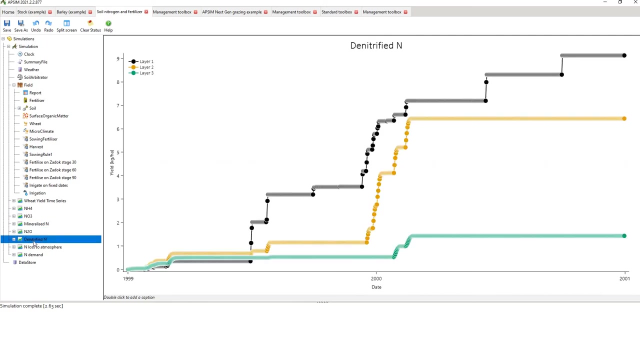 that's then denitrified into nitrate N, which is NO3. you have mineralization, you have nitrous oxide- nitrous oxide is the greenhouse gas lost from the soil. you have denitrified N, you have total nitrogen loss to the atmosphere, and then you have what's an interesting variable nitrogen demand. so 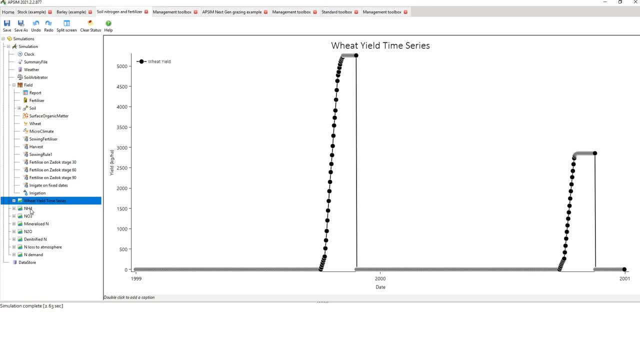 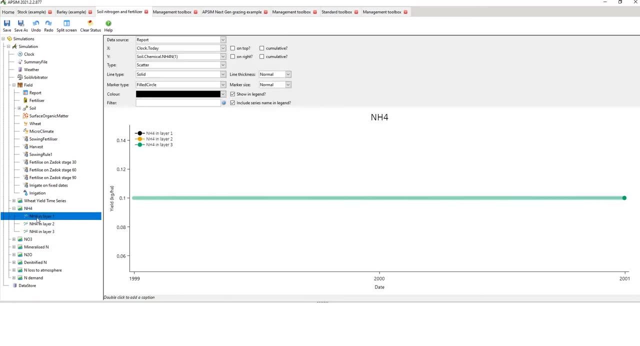 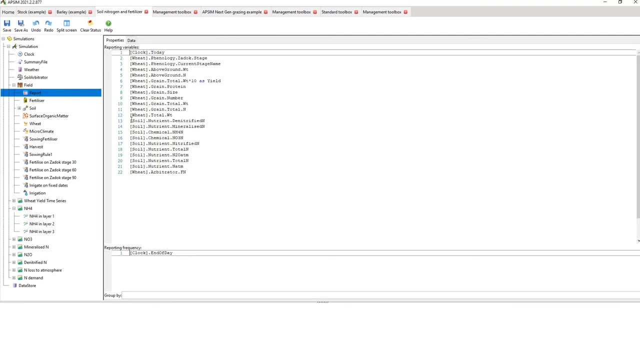 we'll go through these. we've talked about in previous webinars Nitrogen, Ammonium, NH4, so you can plot that in different layers. so I've said so. what I've done back here in the report is you put in your node with 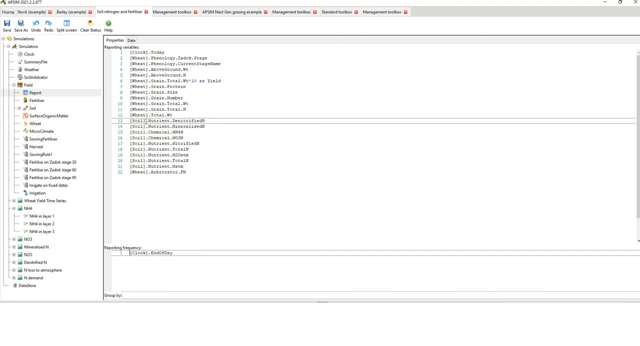 which you're going to get it from. so I've said soil, full stop, sort of the next component that it's going to come from, then nutrient, then denitrified N. If you're not sure how to get these values, how to get these variables, rather you just you put in soil, in square. 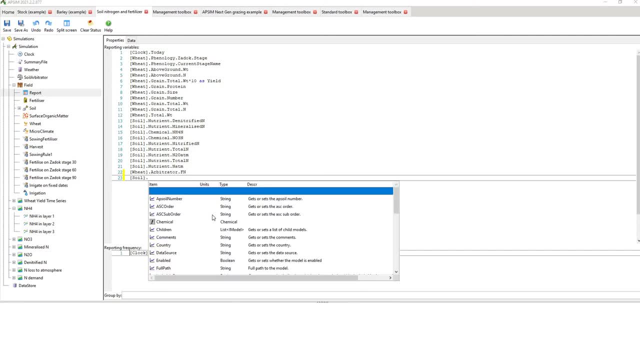 brackets, so that means it's referring to the soil node. you hit full stop and it comes up with a list. so that's quite useful. Then you can double click or you can type it in. so I often double click and then you hit full stop again and it comes up with a secondary list and it actually says the units. 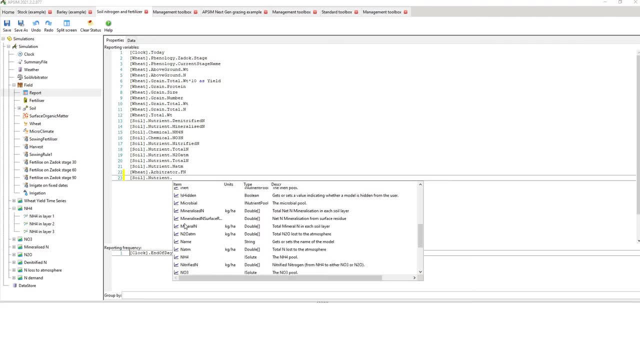 and the description of them, which is very useful, so you might want to have a look at those. So there's a bunch of different nitrogen out there. So that's how you determine what variable you're actually looking at or what variable you can plot. 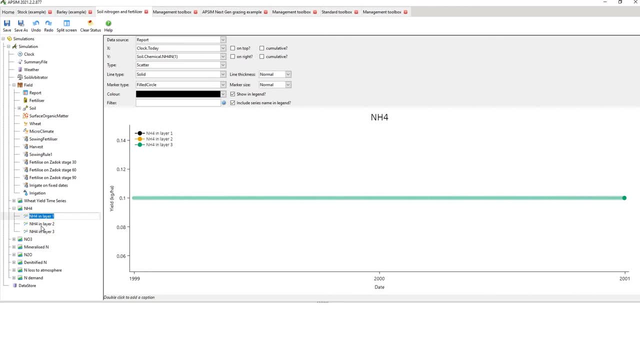 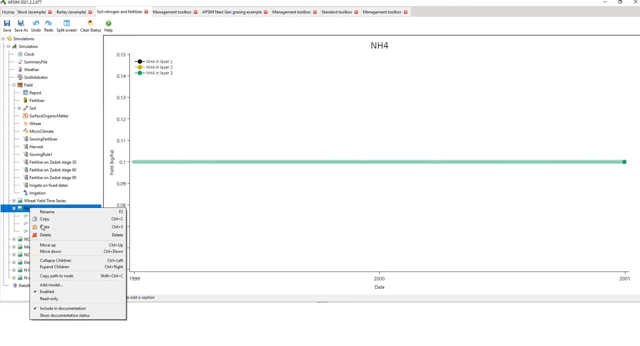 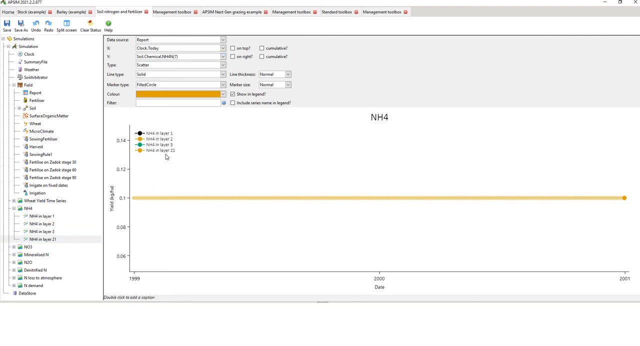 And then you can copy this and put it there, so drag it up and drop it on the top level so that it actually comes up again. so if you copy that and paste it on there, you bring up another level and you might want to say: I want to look at nitrogen in level 7, ammonium. 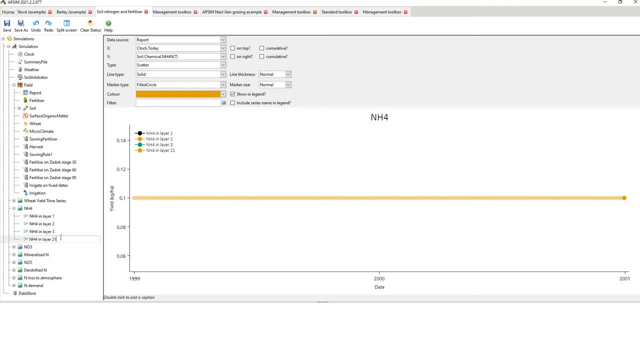 in level 7.. And so you have to change the label manually. so I just encourage you to do that. so here you can see that that label is actually wrong. that should be ammonium, not yield. that's just a residual thing. I've copied the graph above. 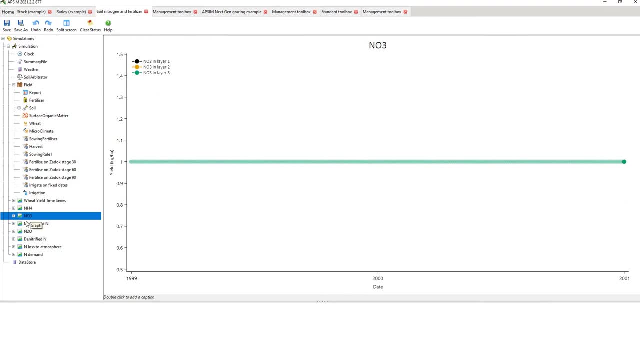 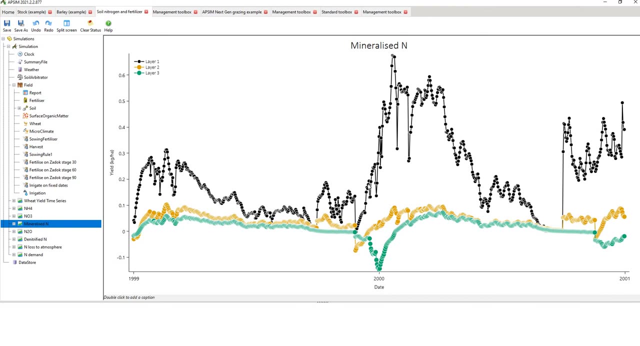 So we have the same thing for nitrate. you can see nitrate is static Mineralised N, so I've plotted it in only the first three layers. you can see that what's happening here is we're getting large variability in nitrogen mineralisation in the top layer. 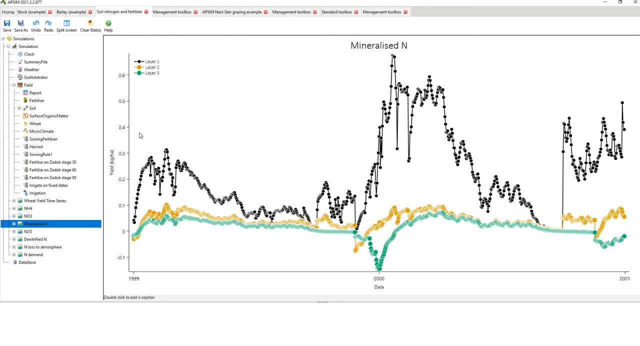 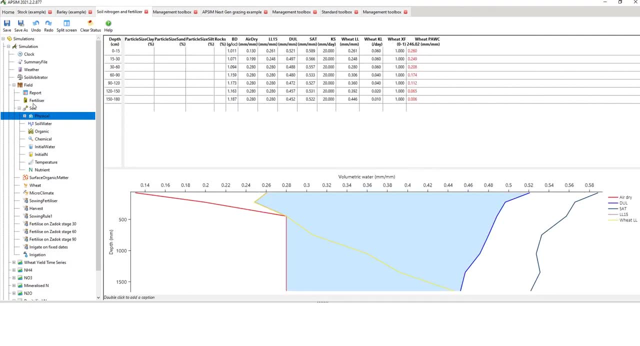 not so much variability in the second and the third layer. so you might say what are the second and the third layer? you can go back here to the soil and you can actually see what depth they are. so 0 to 15,, 15 to 30 and so on. 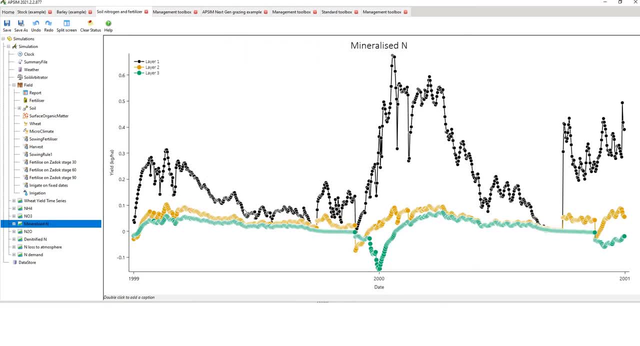 So that's your mineralised N, which is quite useful. The crop is growing in this season, so this is winter and you're not getting much mineralisation. you're getting a lot of mineralisation in summer, and the reason for that is because not only warmer temperatures, but I applied irrigation around about this October period.